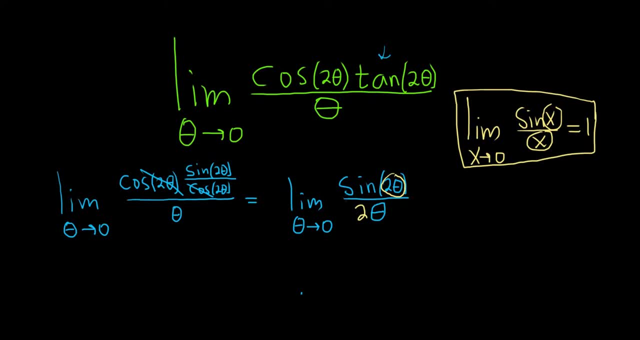 All right, we can just put it there, But we can't really do that unless we take it away. So I'm going to put it, I'm going to put it up top as well, like this: Let me see, And now what you can do is you can pull this two out, So you can write it like this: 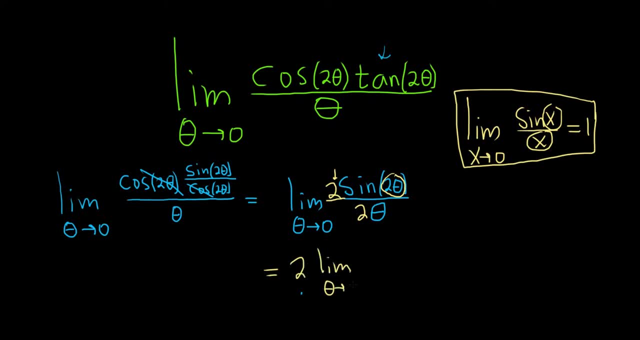 Limit theta approaches zero of sine two theta over two theta. And now you see it matches. It matches just like the formula does. You see you have the x and the x in the formula. Here you have the two theta and the two theta And as theta approaches zero, two theta approaches zero. 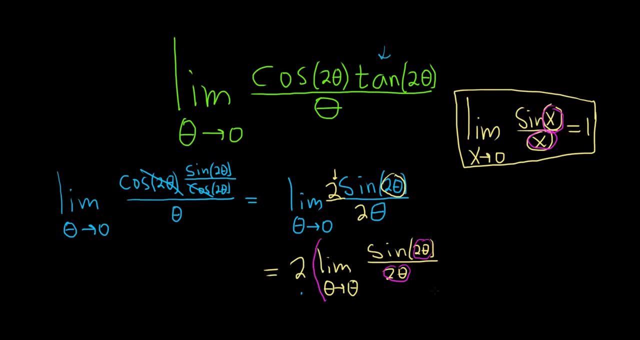 So it matches the formula formula. so this piece here in parentheses, it's going to be equal to 1 from the formula. so it's 2 times 1, so that's equal to 2 and that should be the final answer. so very important to you know. carefully, show the work here. I. 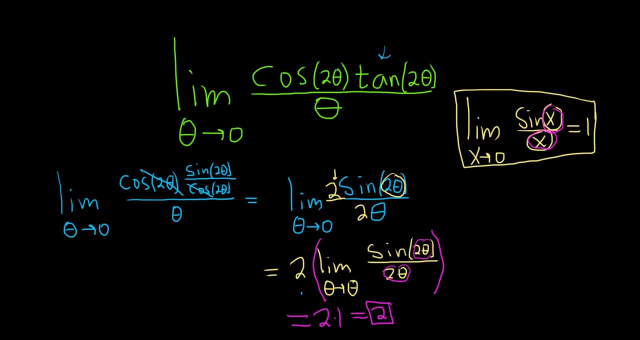 usually don't don't do it like this. usually I usually go from from here to here. so I, if it was, I would just do this. if it was me, I showed an extra step there and then I put the 2 theta on the bottom, you see, and then you can just see. 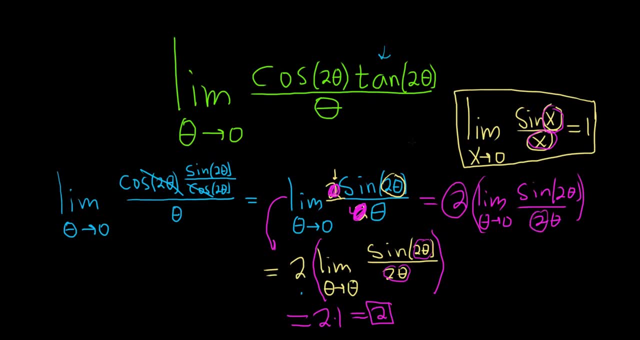 you know that these cancel. right, this one and this one cancel, so we really just get this. so, and then from here you just do 2 times 1, so it's 2. I hope this video has been helpful.